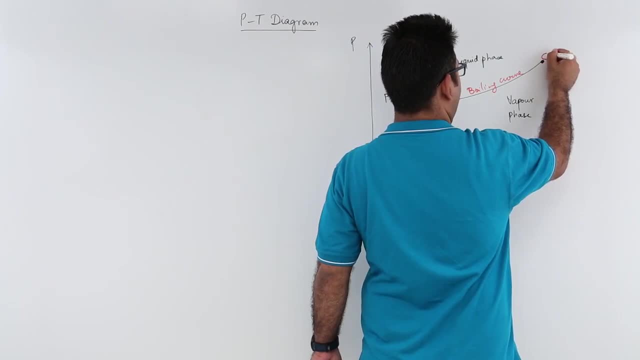 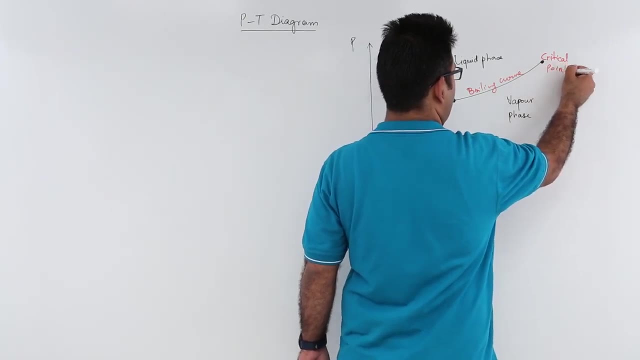 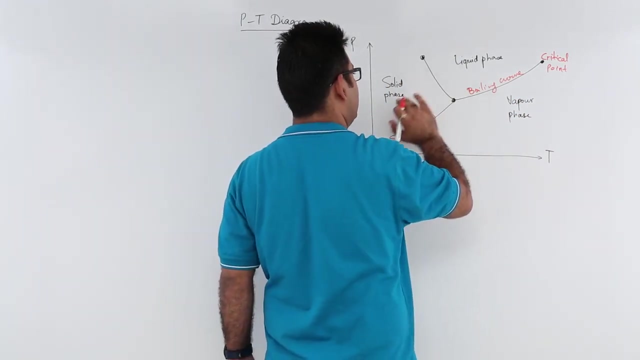 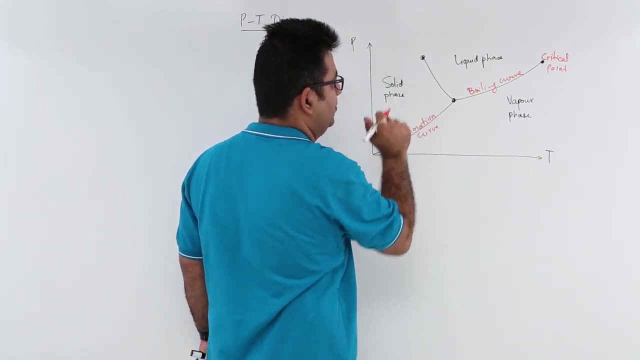 And this point is called the critical point. This is the critical point where there is almost no distinction between the liquid and the vapor state. Okay, Now you see this conversion, that is, the solid to liquid conversion. Okay, Let us take the case of ice, because it is showing you a negative slope. 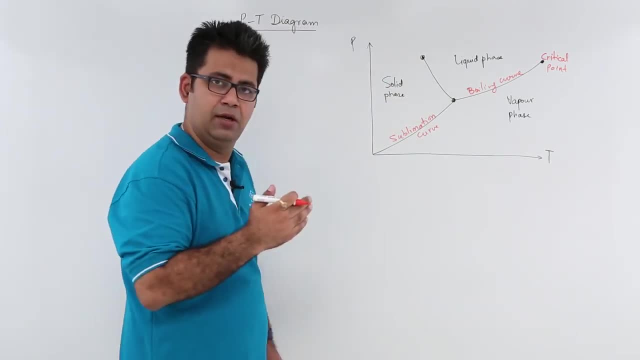 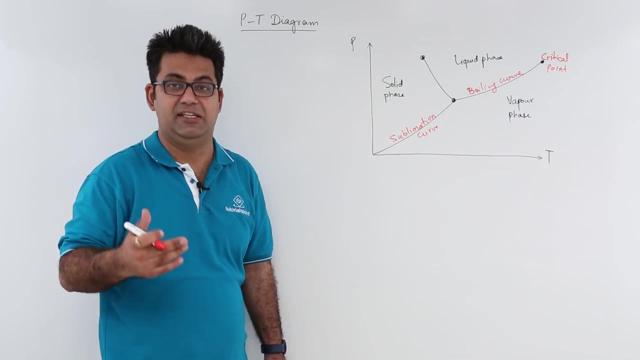 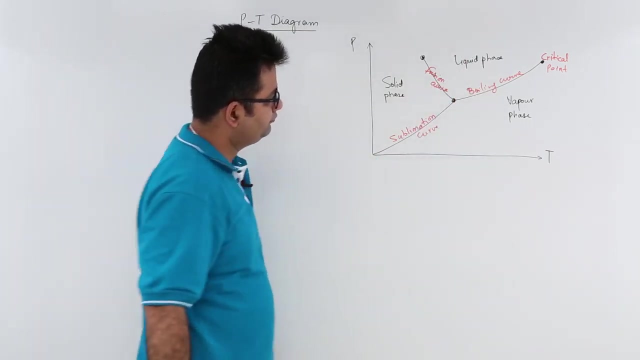 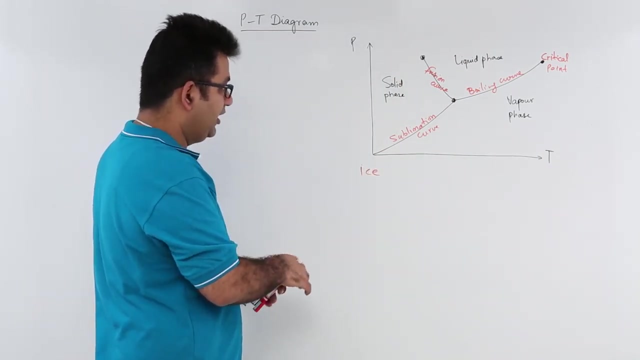 Which means as you increase the pressure, As you increase the pressure or the saturation pressure, the saturation temperature decreases. That is for ice, So this is called the fusion curve. Fusion curve- Okay, So this is specifically for ice, Which shows that upon increasing the P, 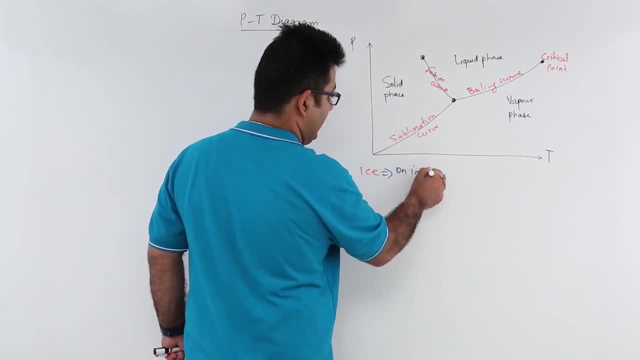 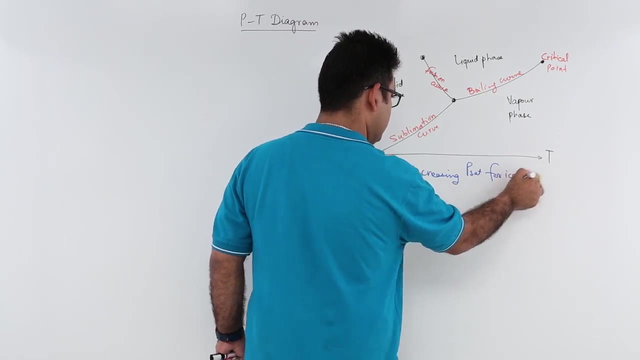 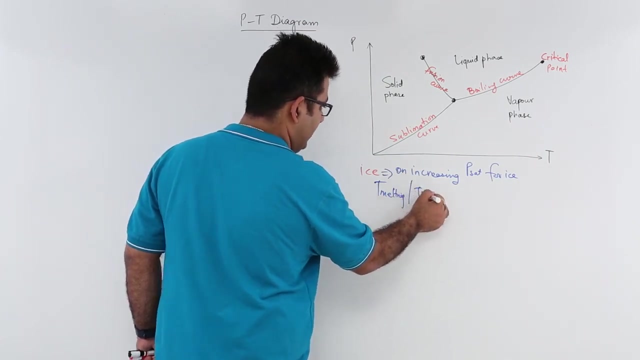 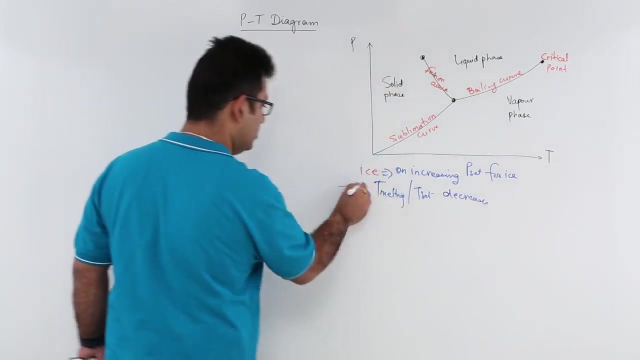 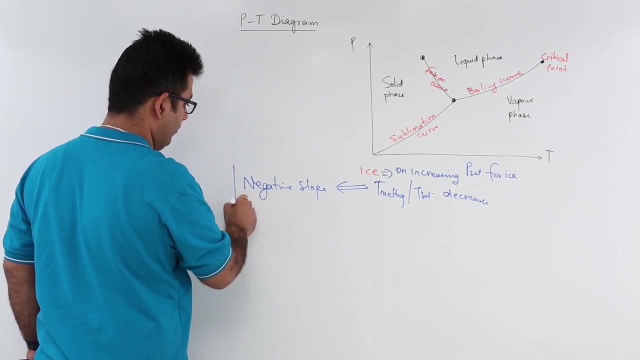 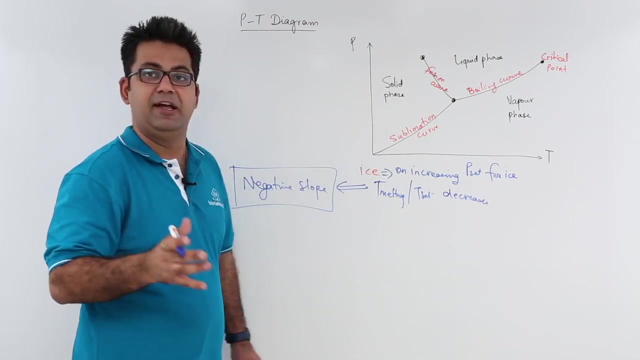 So this shows, on increasing The saturation pressure for ice, Okay, The temperature of melting. The temperature of melting, or this is also called the saturation temperature of the fusion process, It decreases. So this shows a negative slope. Alright, Now you understood this very simple and small, you know. representation of the PT. 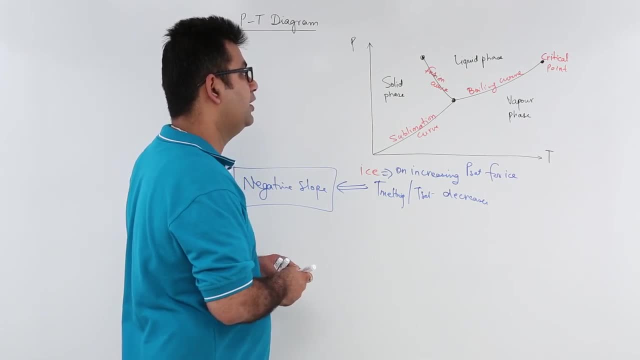 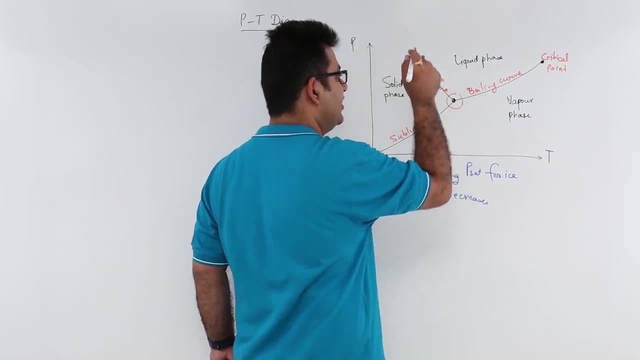 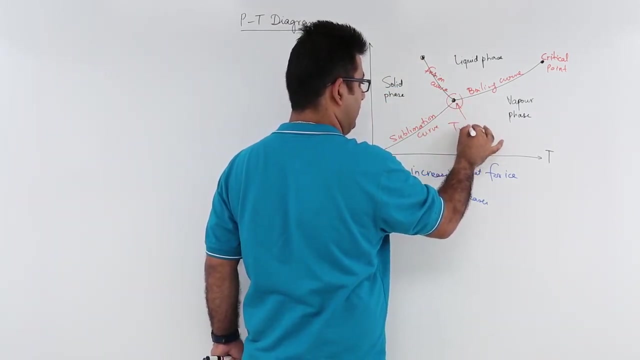 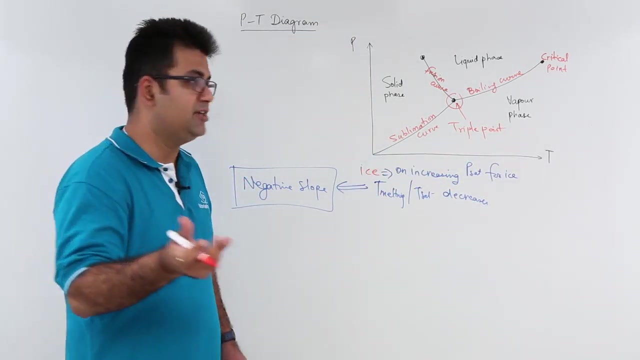 Diagram And there is one more very important point in this particular diagram, Which is this point. So this is the point where the three phases coexist simultaneously, And this is called the triple point. This is called the triple point. Okay, So we have now defined two points. 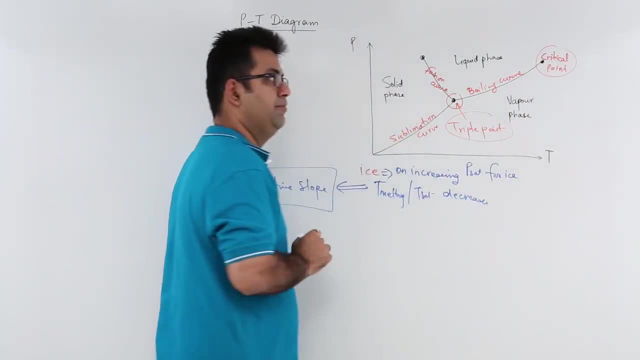 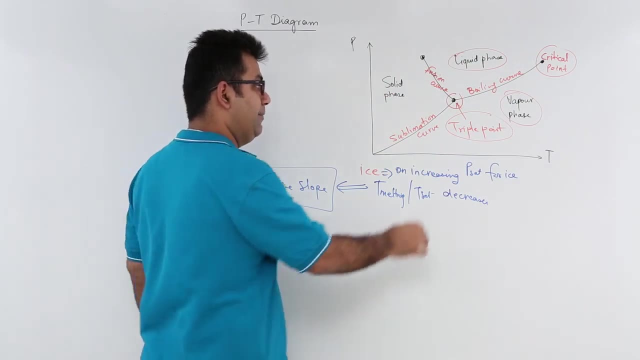 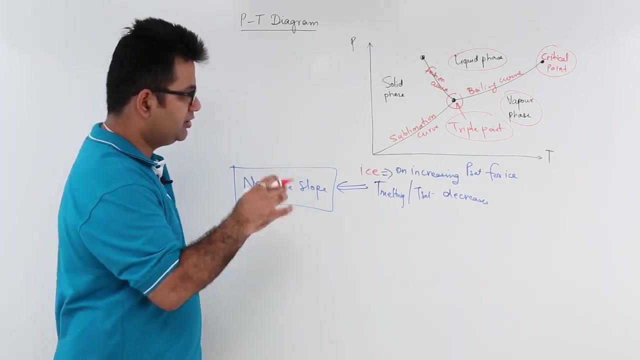 One is the critical point and one is the triple point. Okay, Critical point is that point where there is no distinction between deeper and vapor phase, And triple point is that point where the three phases coexist simultaneously. Okay, So this is all that we have to understand in the PT plot. 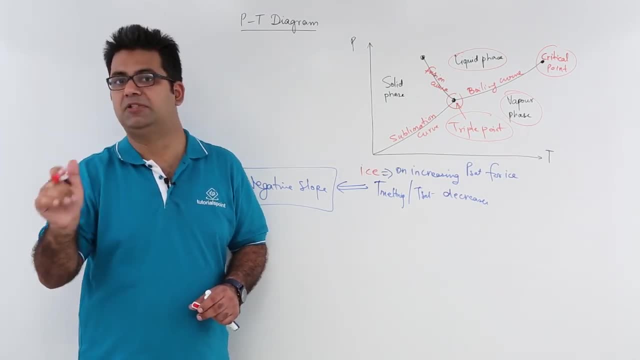 Now let us understand the PV diagram in the next video. Okay,